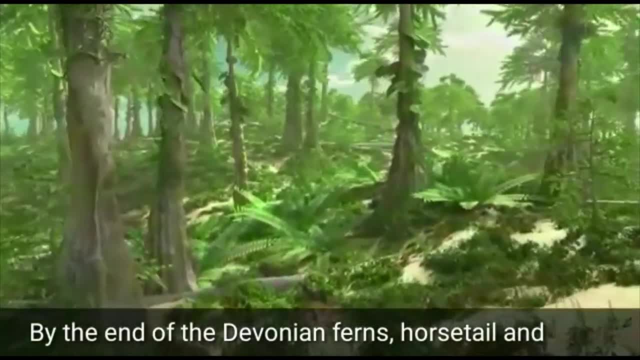 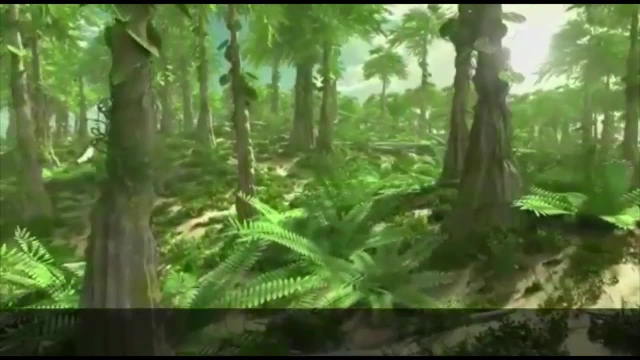 By the end of the Devonium ferns, horsetails and seed plants had also appeared, producing the first tree. By the end of the Devonium ferns, horsetails and seed plants had also appeared, producing the first tree And the first forest. 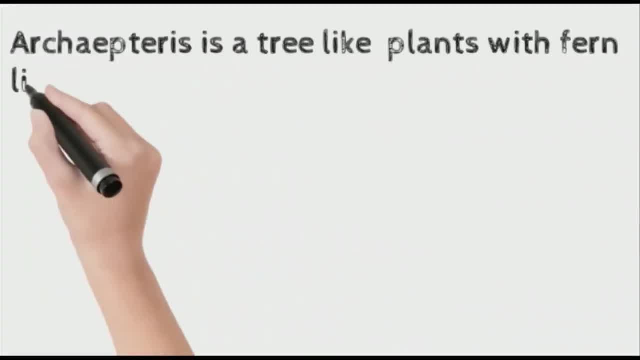 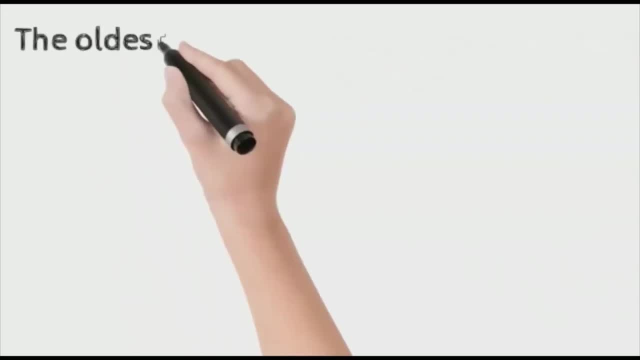 Archaeopteris is the tree like plant with a fern like leaves and the first forest. The oldest fossil of this type of plants is found 385M years ago and has global distribution. Archaeopteris was the first15- persistence thinker that invented. 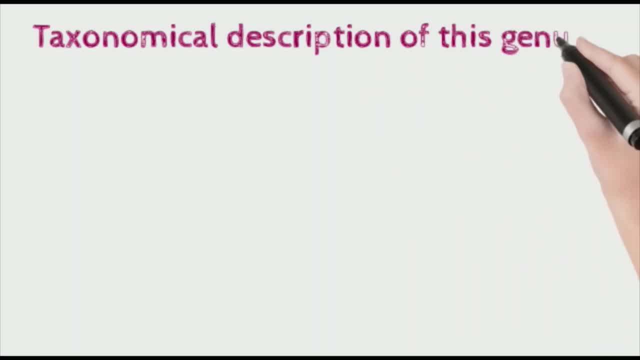 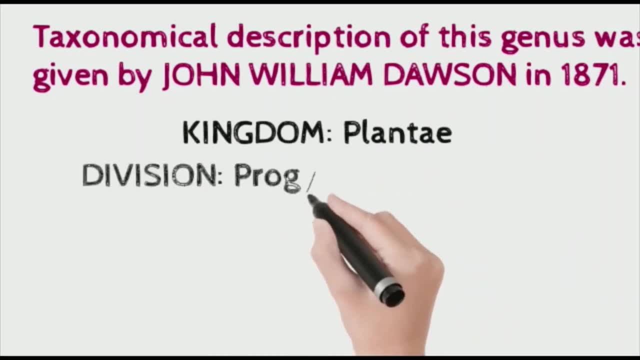 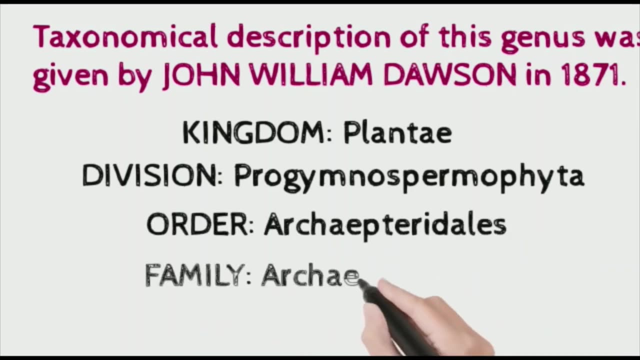 The first exinomical division of this genus was given by John William Dawson in 1871. By the end of the Devonium, ferns, horsetails and seed plants had also claws. likeooky letter 258V as Kingdom Plantae Division Progymnospermophyte Order Archaeopteridales and Family Archaeopteridaceae. 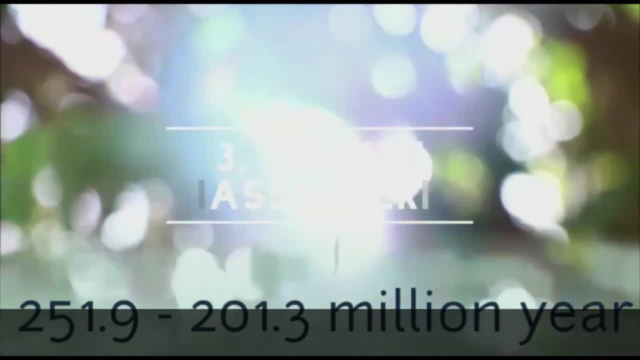 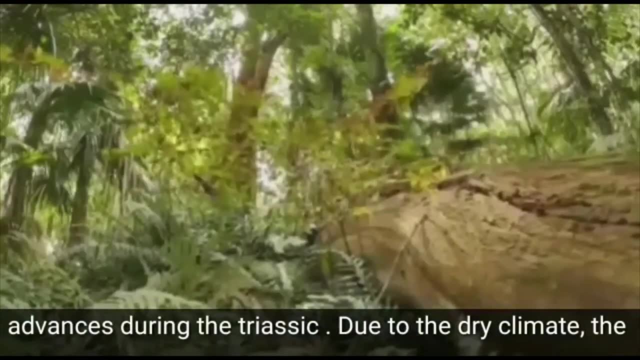 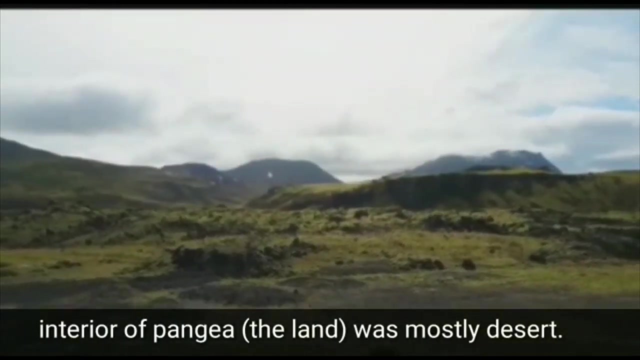 The next plant in this series is from Triassic period. ie Zomite Plant did not go through any extensive evolutionary advance during the Triassic. Due to the dry climate, the interior of Pansrea was mostly desert. Zomite are short plants, look like tiny trees. 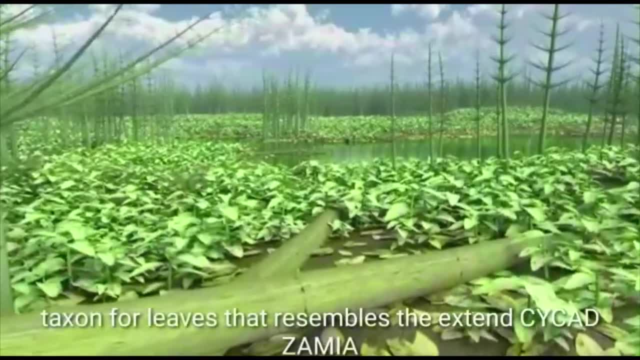 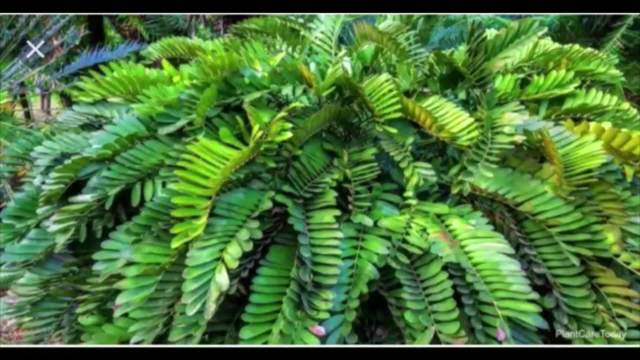 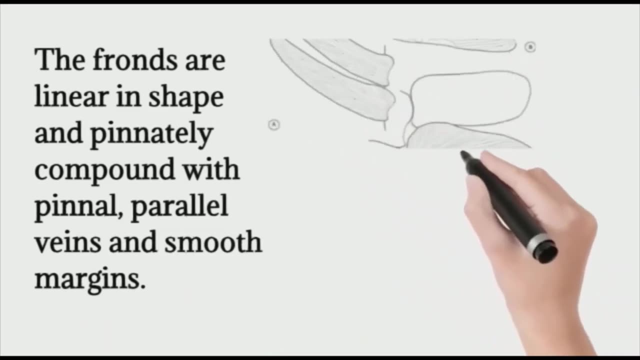 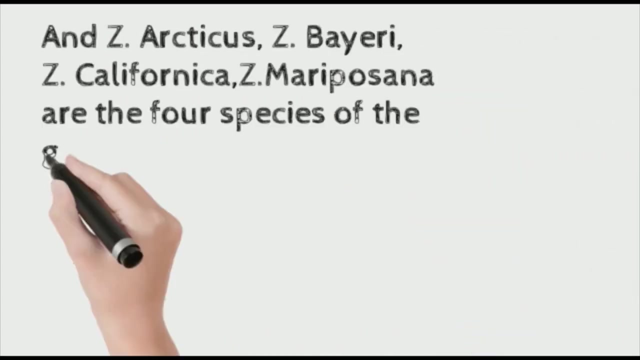 It is a form taxon from leaves that resembles the extant cycade Zomia. The fronds are linear in shape and pinnately compound with pinnal parallel veins. They form a smooth margin. There are four species found of this genus. 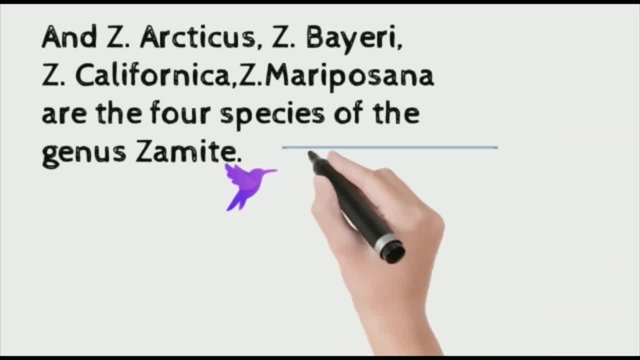 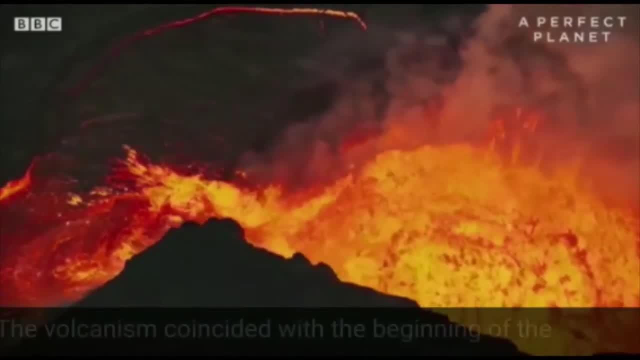 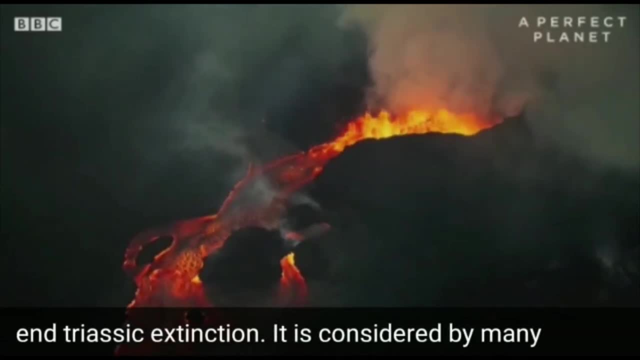 They are Zomite arcticus, Zomite beri, Zomite californica and Zomite mariposanna. The volcanism coincided with the beginning of the end Triassic extinction. It is considered by many paleontologists to be the extinction symbol of Triassic schoning. 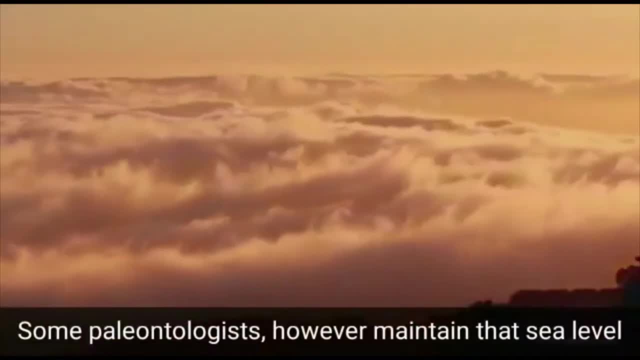 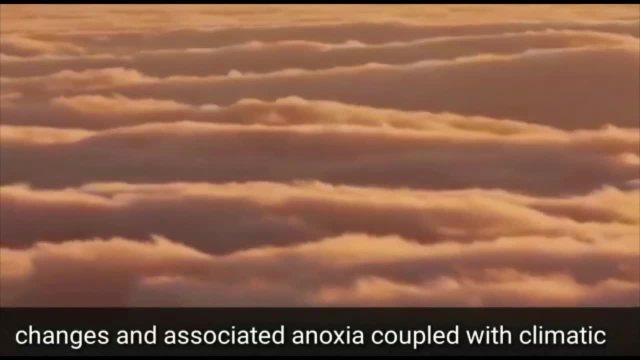 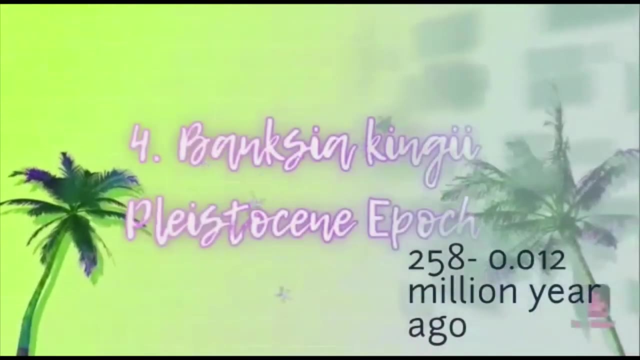 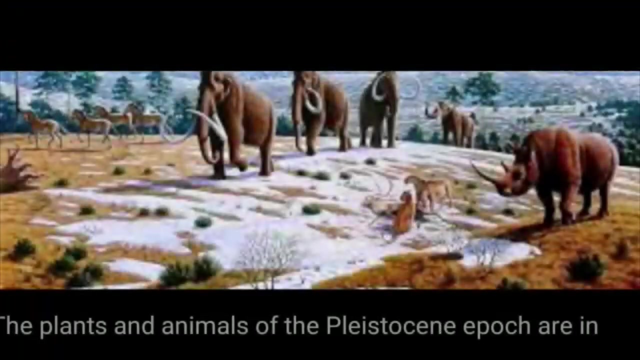 most likely cause. Some paleontologists, however, mention that sea level changes and associated anoxia, coupled with climatic changes, cause this mast extinction. The next plant in this series is Banksia kinji from Pleistocene epoch. The plant and animals of this Pleistocene are: